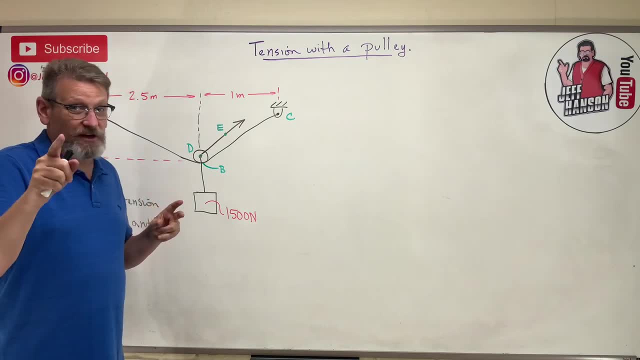 ropes, I'm going to be in trouble. So Johnny Weak Sauce would do that, but not us, right? We're like: no wait, a second Rope goes over pulley. It's the same on both sides. yo, If that equals T. 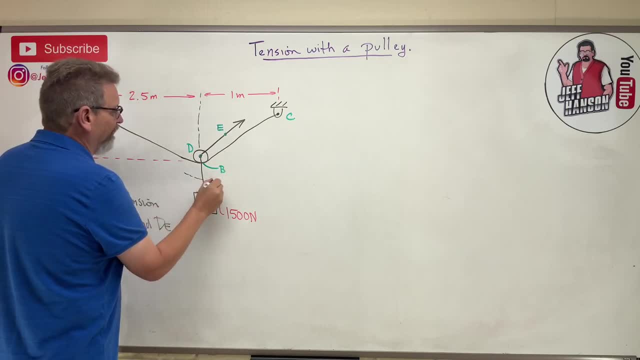 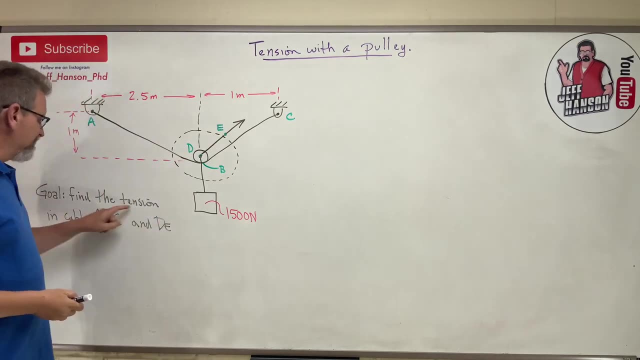 then that equals T. So what I'm going to do? again, free body diagram. I'm going to look at that joint right there- okay, That joint, Because they say: find the tension in cable and they give it to you right here, right A, B, C. What does that mean? That means that this: 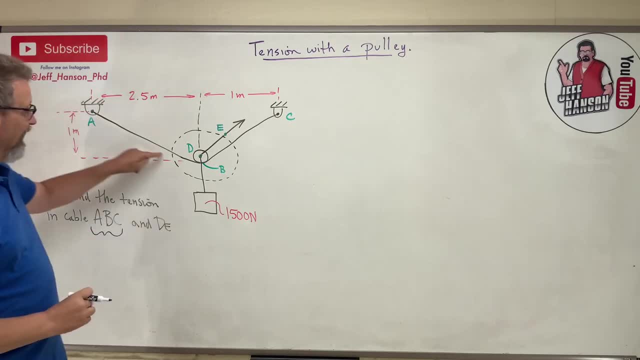 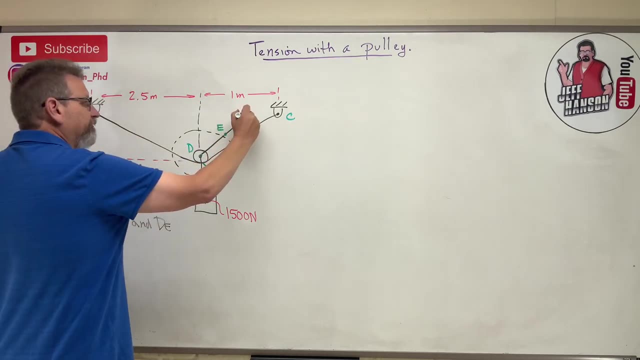 this whole business right, there is all one cable. So A, B, C is one cable, okay, And then D? E is this little guy right here. What is it doing? What is the force? We'll call it force P in rope, D E over there. okay, To keep it in equilibrium. 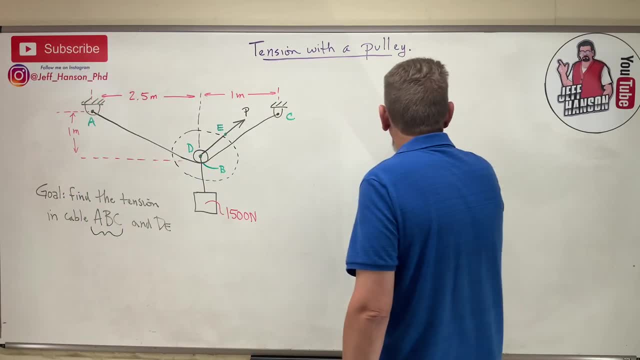 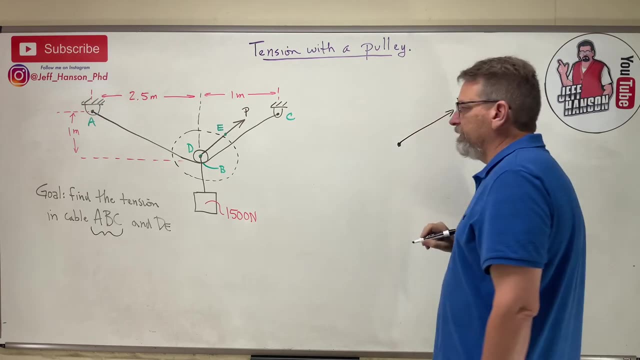 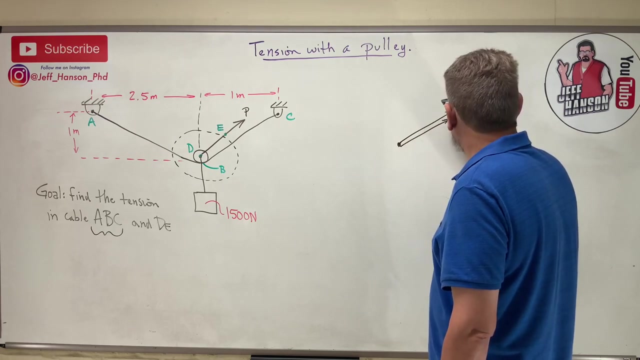 Okay, so here's what our free body is going to look like. We've got that force. we'll just call it F, D, E, okay, And then we've also got in the same direction. I've got force B, C, But you know what? I'm just going to call it T, I'm going to call the tension in this rope. 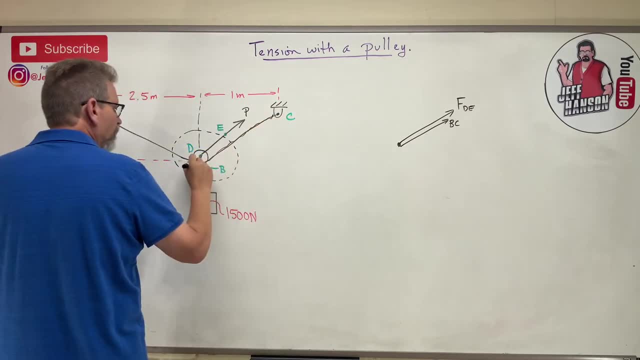 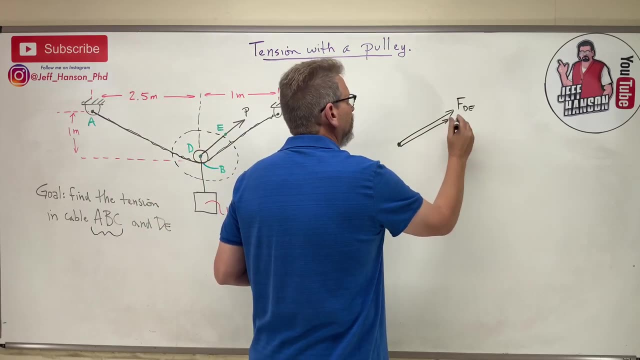 here, right In this one rope, right here, wiggly rope, right, I'm going to call that T everywhere, so it'll be the same, So I don't have different letters there. Okay, I'm going to call U T. 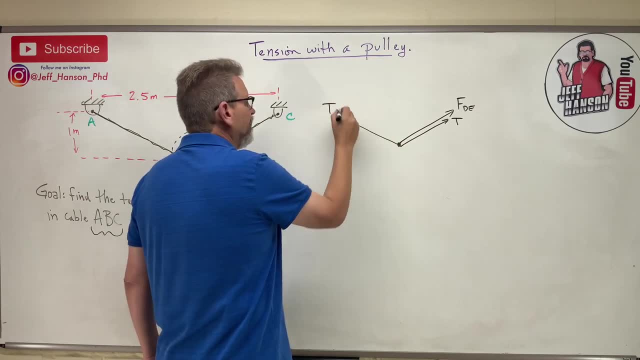 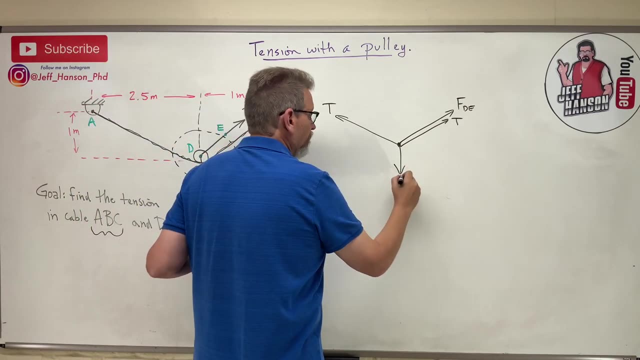 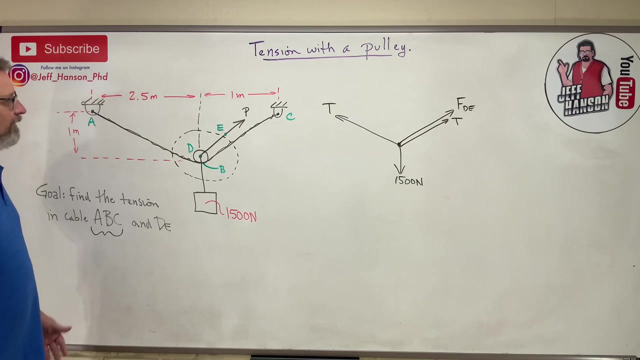 and then this way, there's another T there, and then pulling down on this whole system is our 1,500 newton weight. So the only thing we've got to do here is notice they didn't give us any angles. Well, but that's okay, because we're smarter than the average bear and we're just going to use 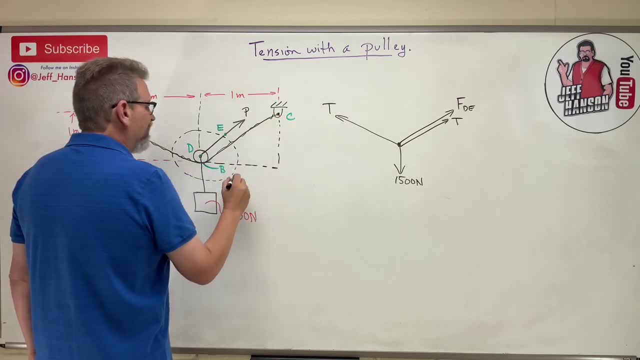 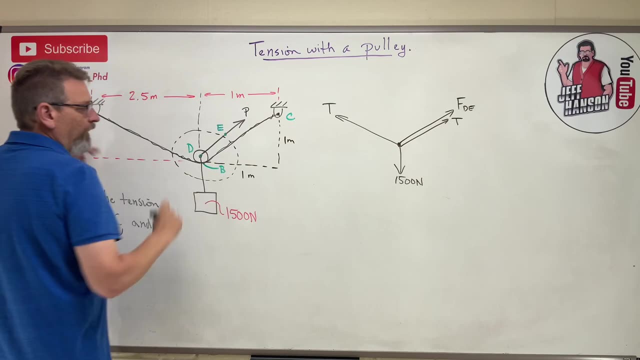 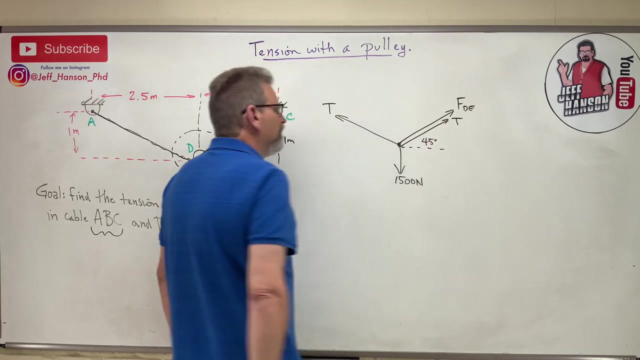 some of these triangles that they gave us here, right? So they gave us that this side is one meter and this side over here is also one meter. So, boom, right now I know that's 45 degrees. yo, All of this stuff right here is at 45 degrees. okay, That's easy. 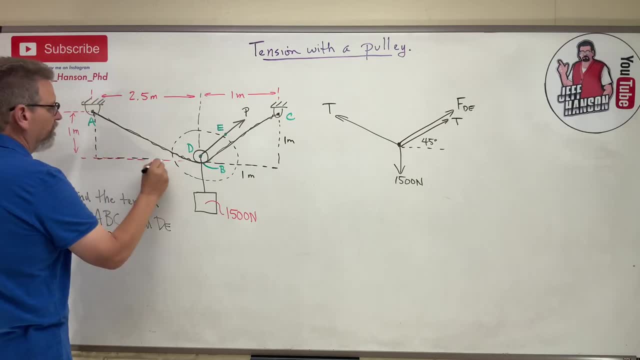 And then I got this guy over here, right, This triangle here which is 2.5 down here and one there. So to find that angle we'll just use a little tangent right. Tan theta equals opposite over adjacent, So one divided by 2.5. 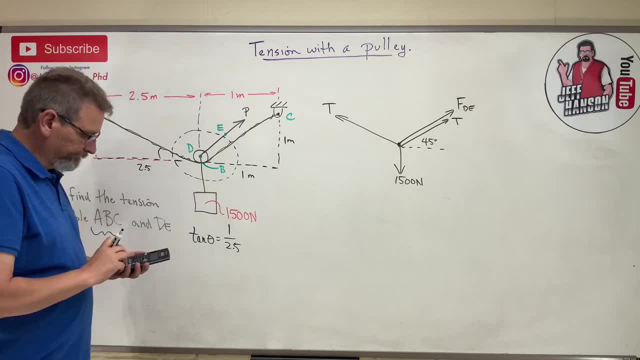 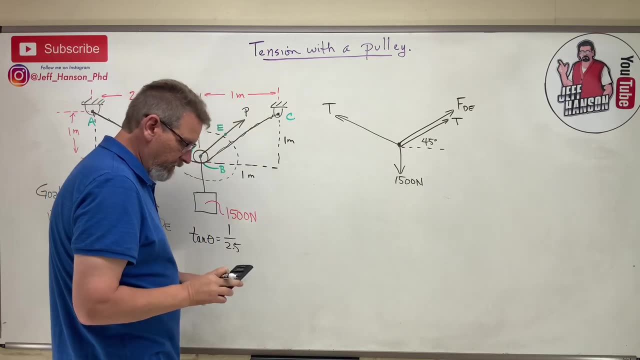 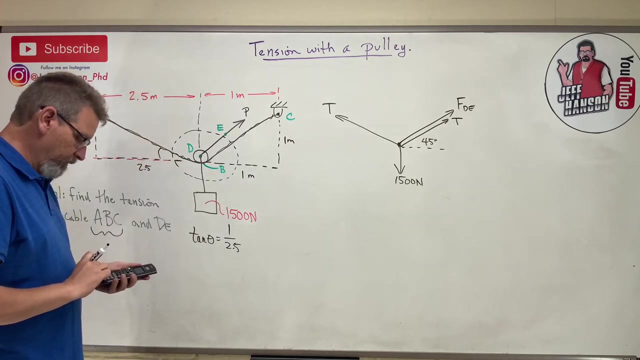 I've got to use my handy dandy calculator. Oh, my handy dandy calculator is no bueno. Okay, Every time I turn it on I have to push the memory clear button for some weird reason. Okay, So one divided by 2.5 equals 0.4, and then the inverse tan. 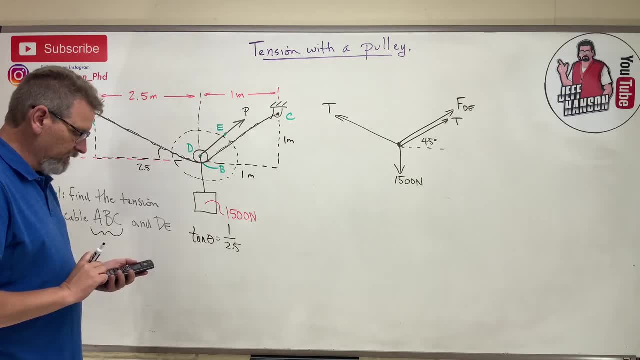 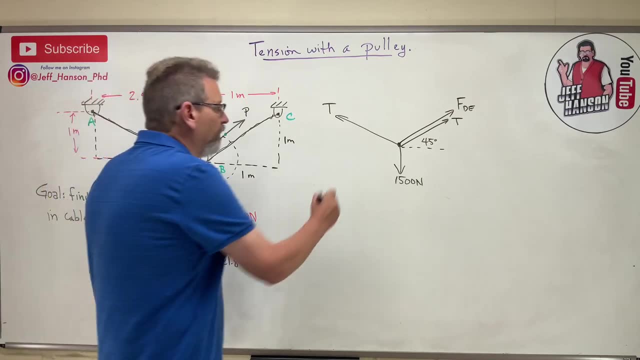 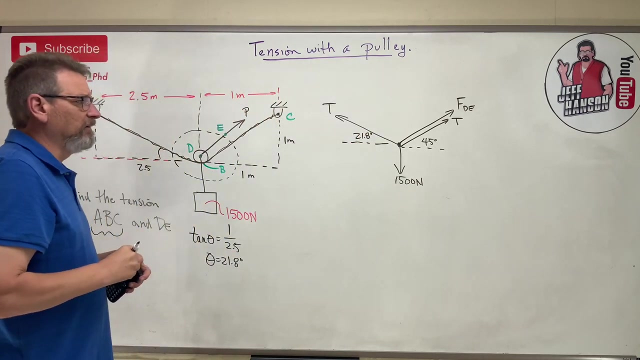 of that is 21.8 degrees, So theta equals 21.8 degrees. So that goes here: 21.8 degrees. Okay, All right, What's left? What's left to do? Well, we've got some vectors and they're at angles, So what do? 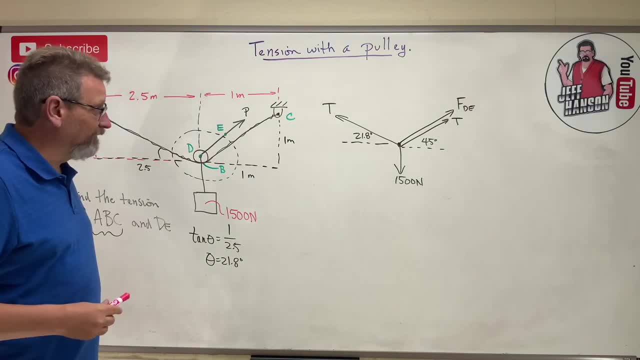 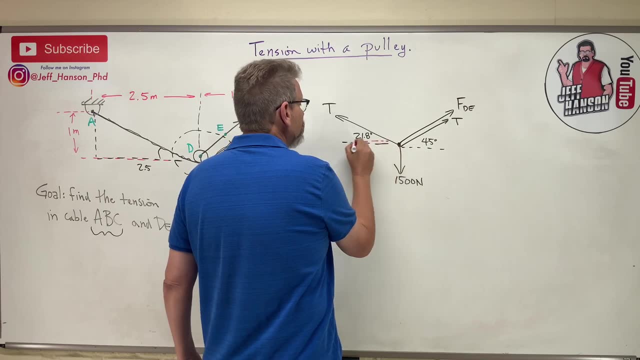 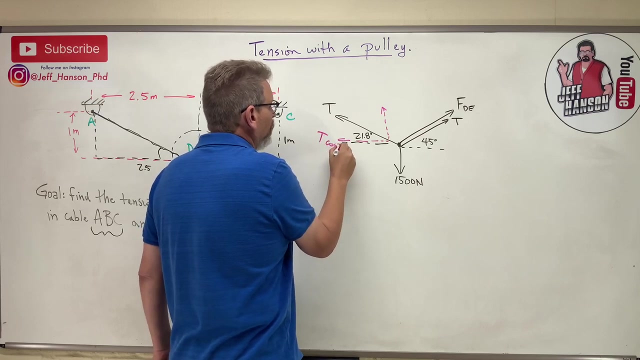 you think By the hundredth time I've said this in these videos. it's time to break it into components. Okay, Let's do it then. Okay, So this guy over here has two components, and they are t cos 21.8. 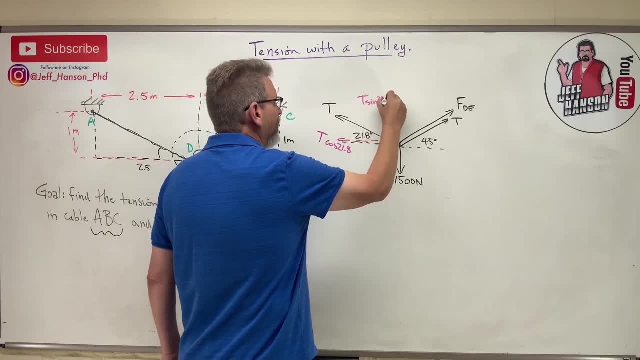 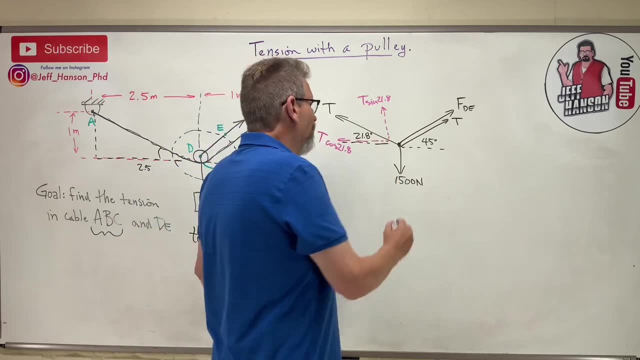 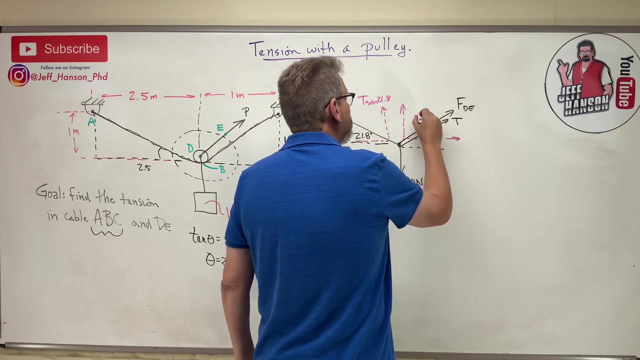 and t sin 21.8.. Now over here it's a little tricky because I got two cables. They're pulling in the exact same direction, So the f cable is going to have one here and one there and the t cable is going to. 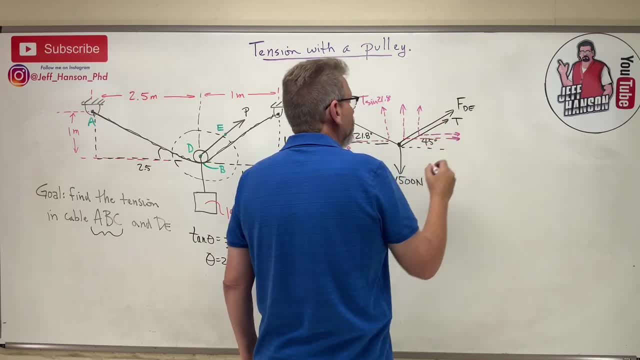 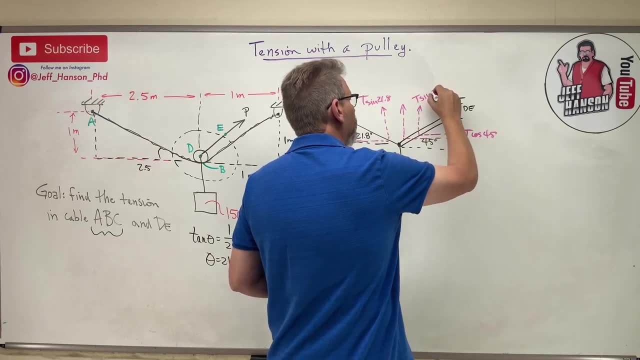 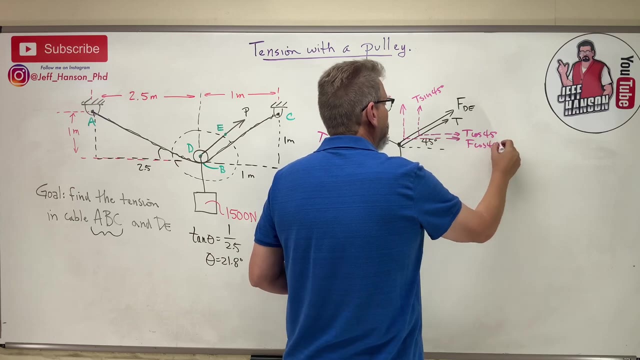 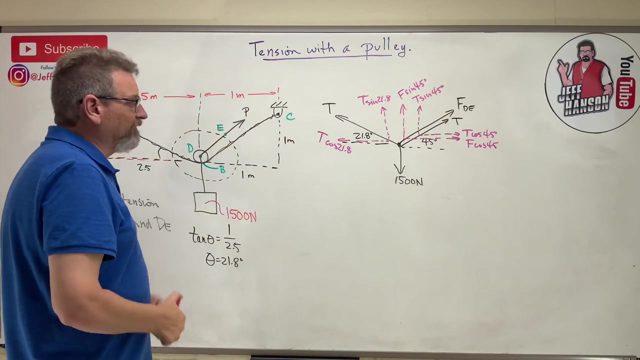 have one there and one there, Okay, So the t cable is going to be t cos 45 and t sin 45, and the f cable is going to be f cos 45.. 45 and f sin 45.. Okay, So now that I've got those labeled, man, how easy is this going to be now? 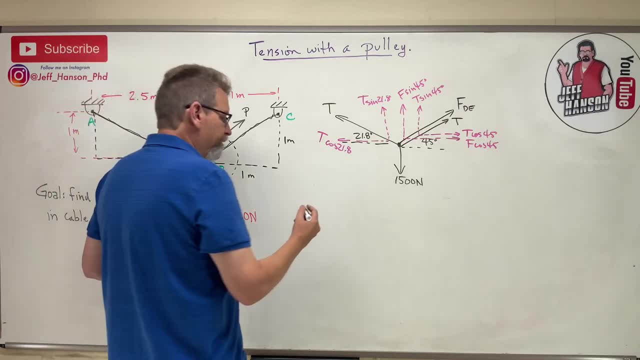 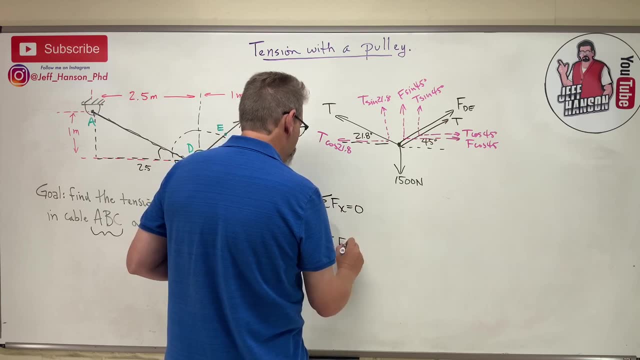 If I can find my pen here, it is right here, Okay. Sum of the forces in the x. Sum of the forces in the y. Okay, Here we go. Let's do the x first. I'm going to do the positive. 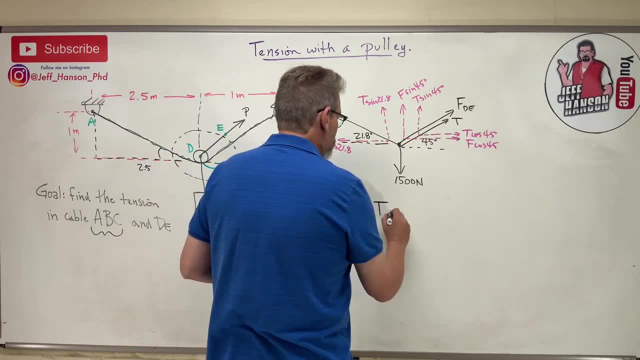 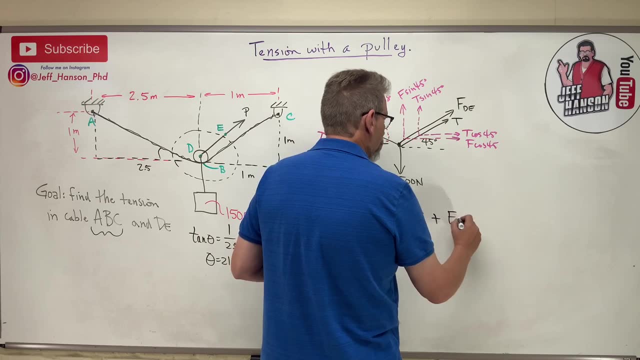 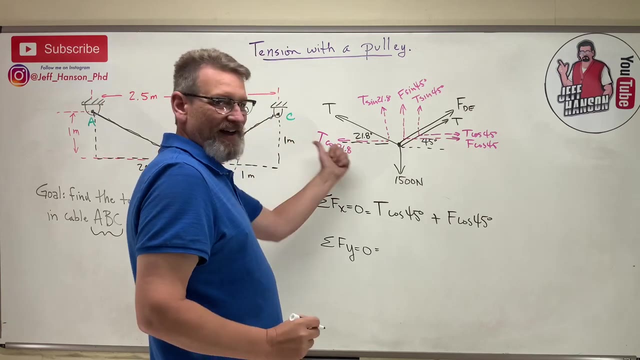 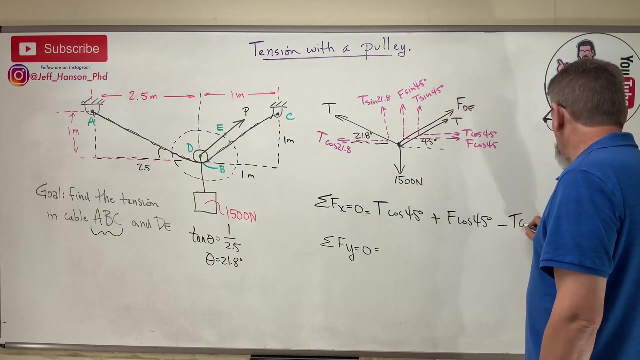 ones. first I'm going to do those two guys: T cos 45 plus F cos 45.. Is there anything else? Oh yeah, this guy over here is the negative x, this guy. So minus T cos 21.8, okay. 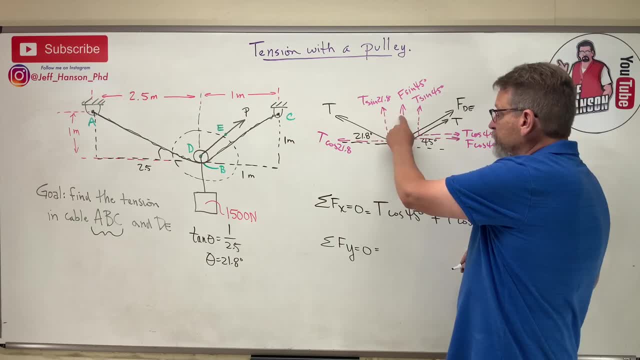 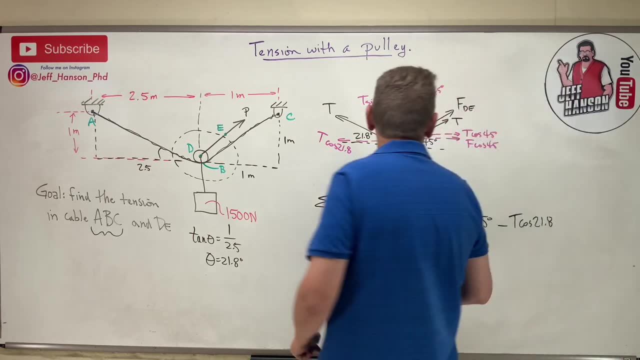 Now I've got to do the y's, so I've got three uphill guys- one, two, three- and I've got one downhill guy, so he's going to be negative. I'm trying to keep my order the same, so I'm going to do this. 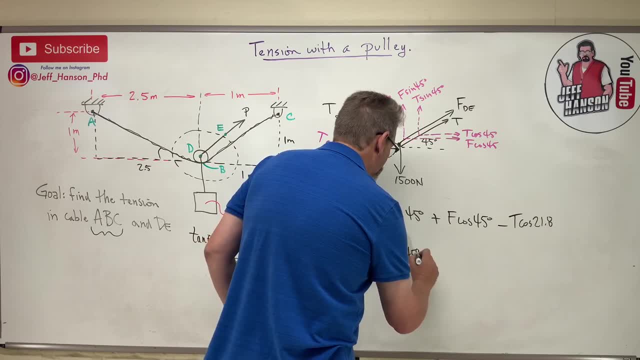 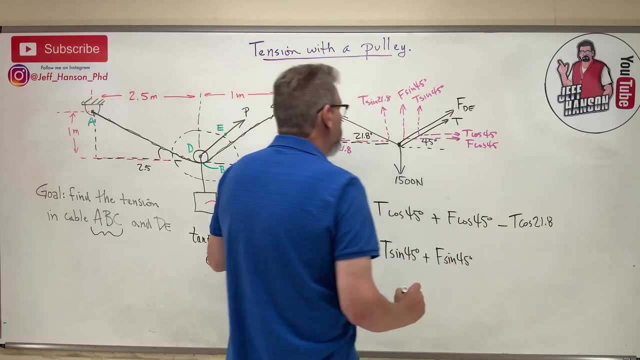 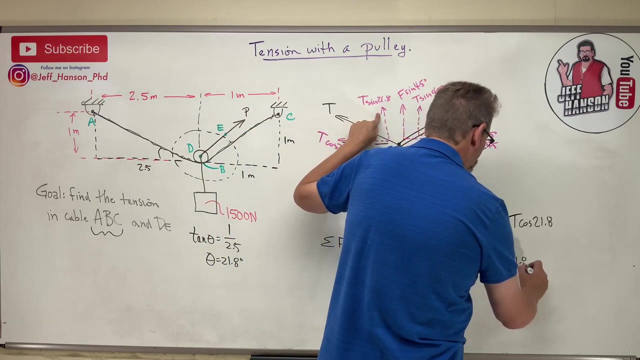 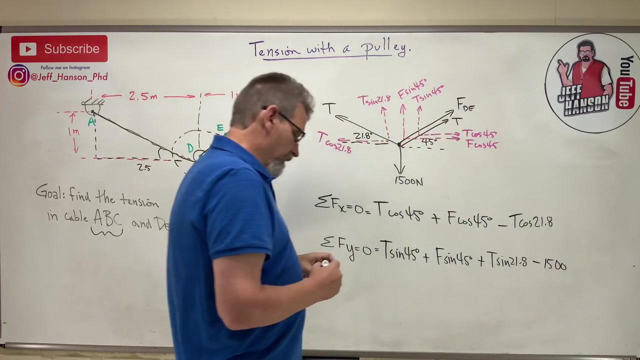 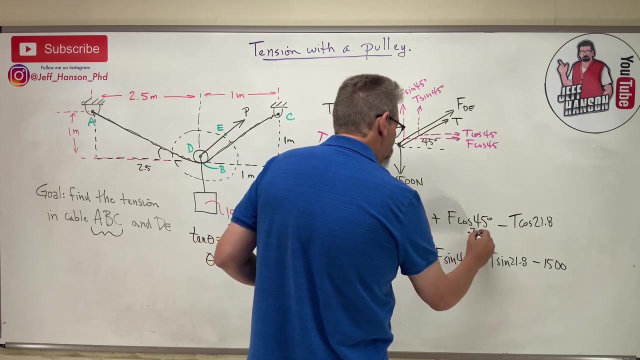 T sin 45 plus F sin 45 plus T sin 21.8, and then minus the 1,500.. Okay, now there's some things I can do here. I know that the cos 45 is 0.707,, that guy's 0.707.. 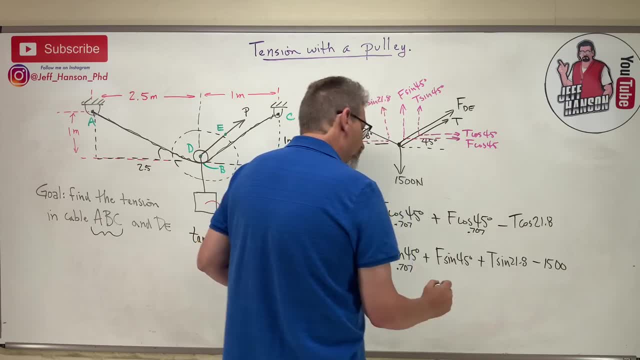 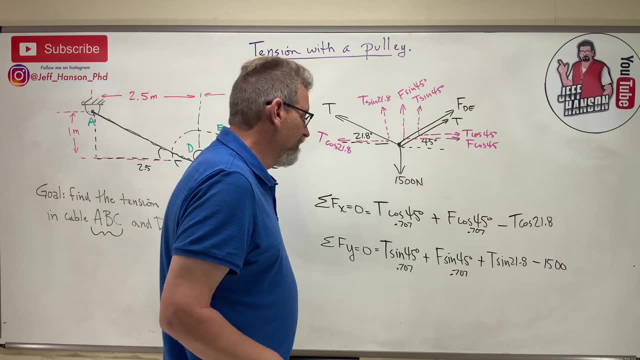 I know that this guy's 0.707, and this guy's 0.707.. I don't know those other ones off the top of my head, so let's calculate that, Okay. so clear, clear, clear, clear, clear. clear. 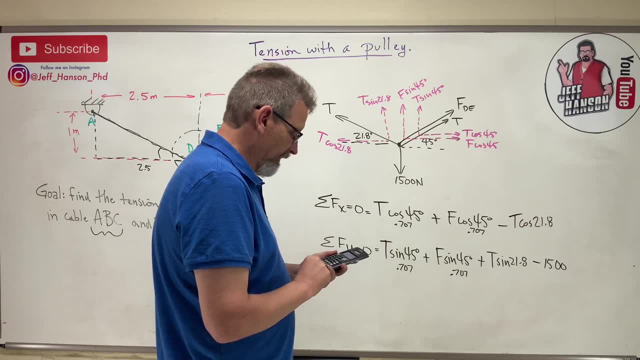 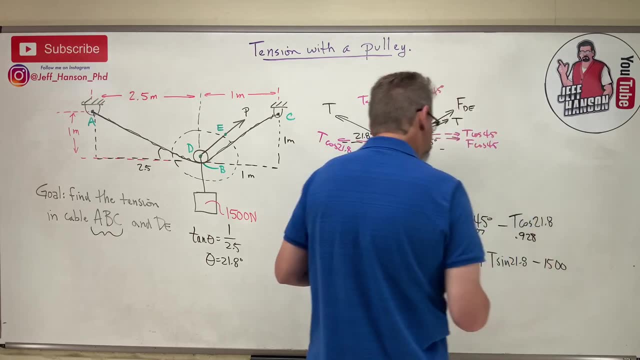 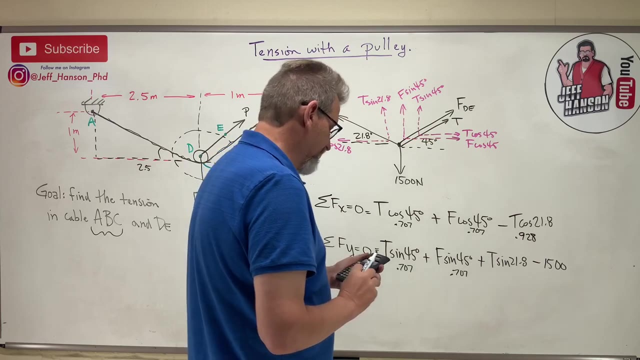 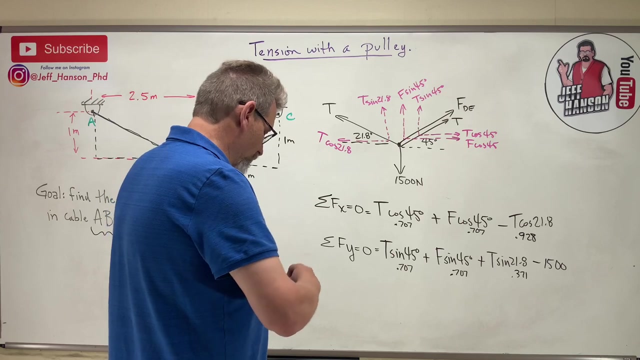 Cosine of 21.8 is 0.928,, 0.928,, okay. And then the sine of 21.8 is: how much is that? 0.371.. So what do I have here? Let's just I'll rewrite these equations in a different color. 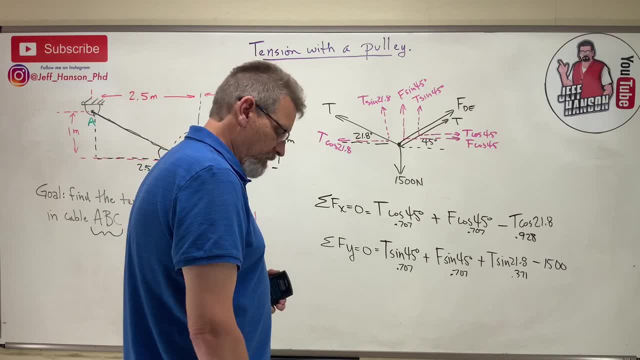 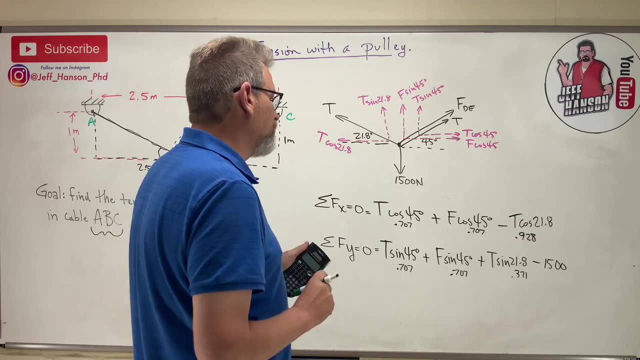 and kind of clean all this up a little bit. okay, What color's going to come out of my pocket? Green, okay, here we go. We're doing it in green Ready. What I'm going to do is combine these two t's together. 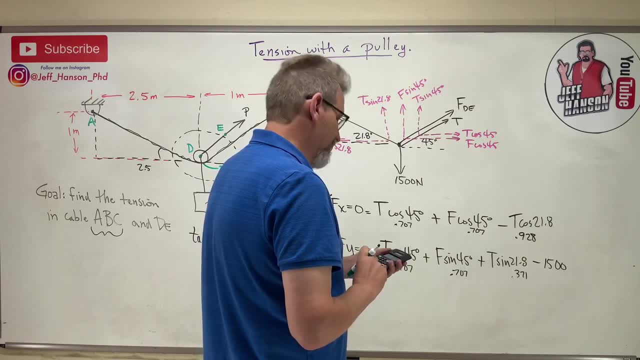 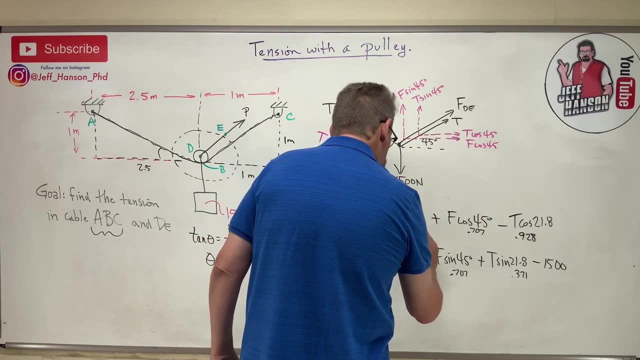 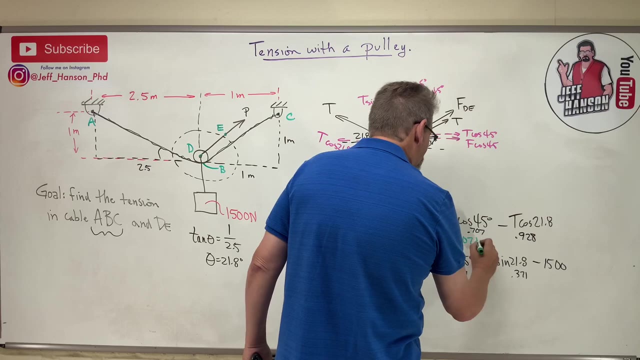 So 0.707 minus 0.928 is negative 0.221.. So negative 0.221t plus 0.707f equals to 0.. There's one equation, the green equation. right, Let's clean this one up, okay. 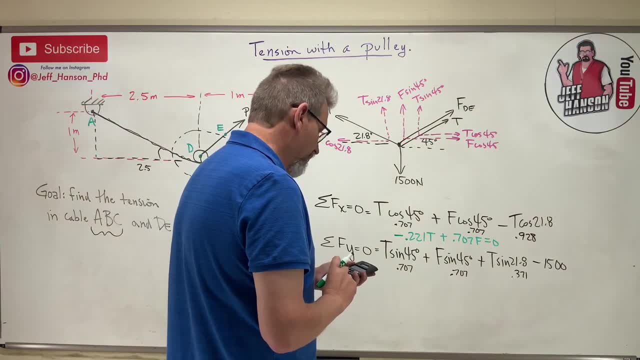 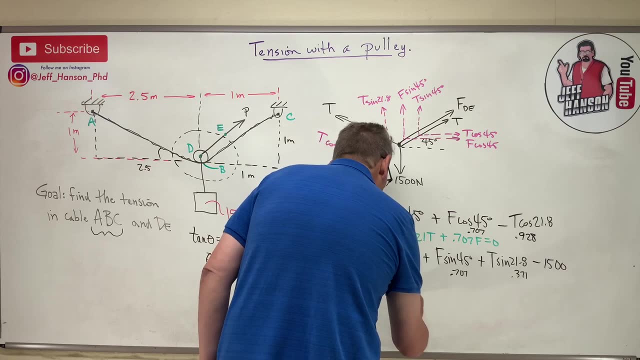 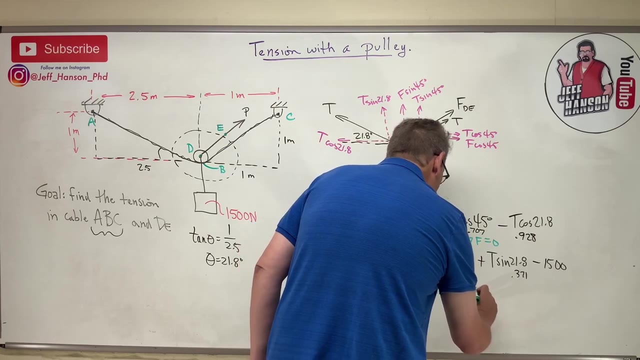 So 0.707.. 0.707, this time plus 0.371, 1.078.. So 1.078t plus 0.707f and I'm going to move that 1,500 to the other side. 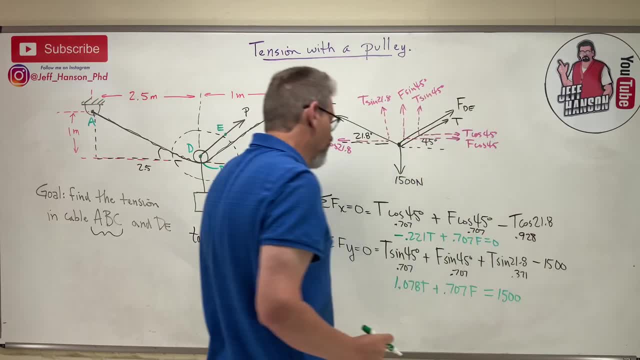 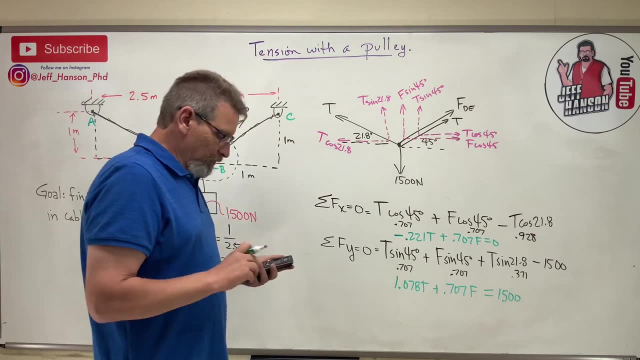 equals 1,500.. And look what I have now. I have two beautiful equations: The t's are in line, the f's are in line, the constants are in line. Dude, I can use this, I can use my system solver. 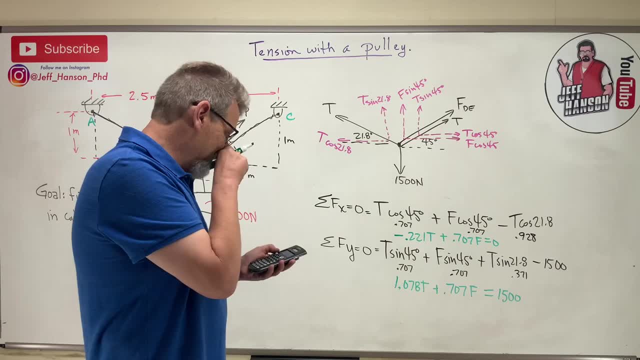 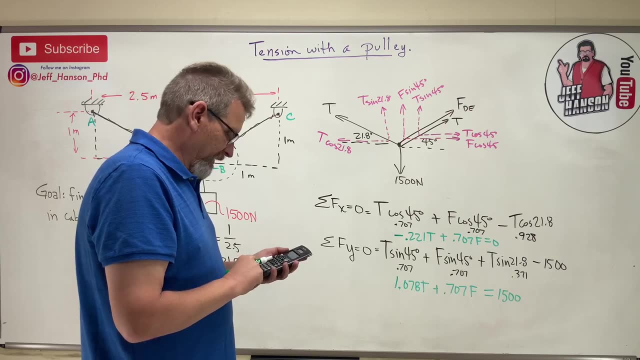 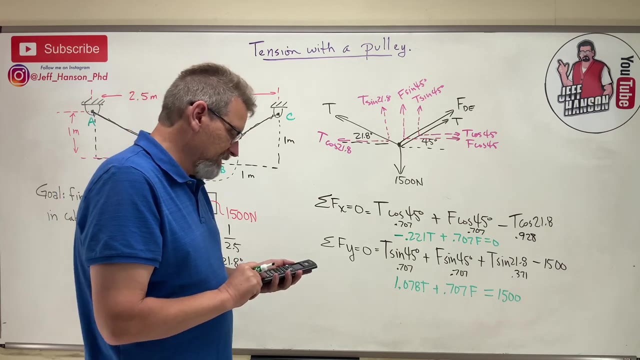 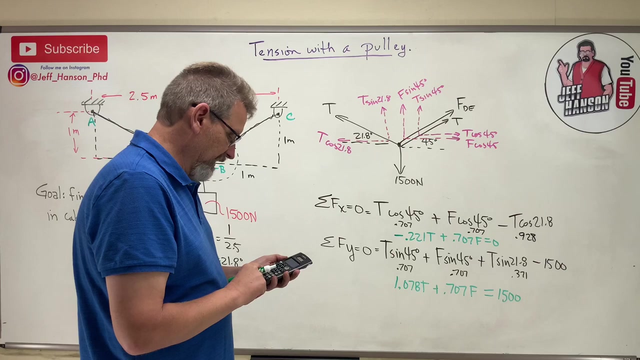 Watch this, This is no problemo. Okay, so I'm putting this in Negative: 0.221, enter- enter. 0.707, enter, enter, enter And then 1.078, enter- enter, 0.707, enter and then 1,500, enter. 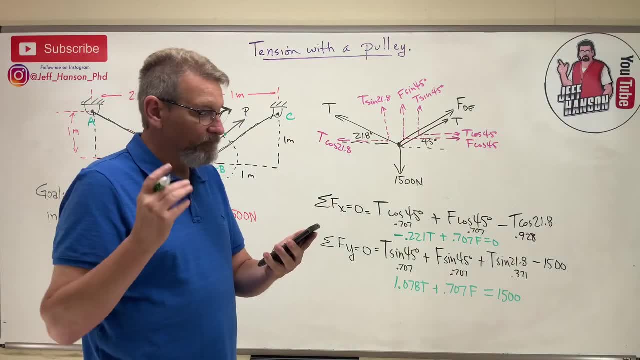 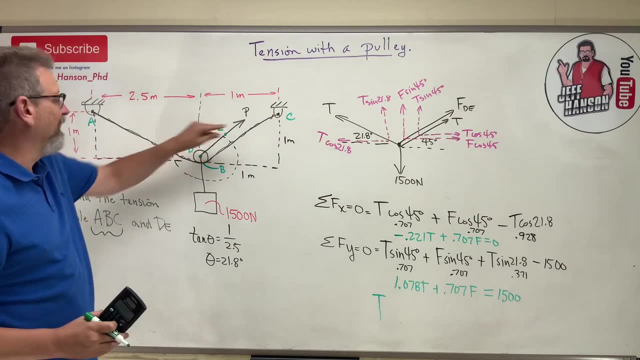 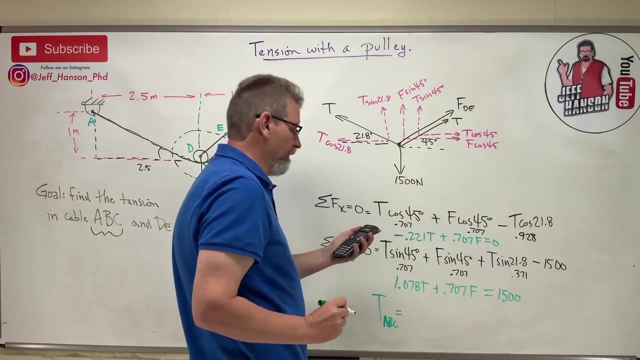 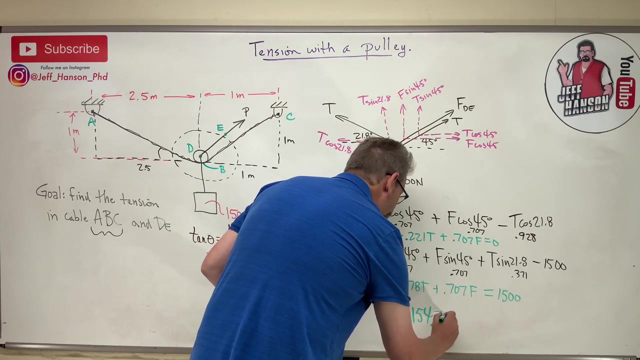 Now I'm on solve. Solve boink done. How easy is that? So t, which is t a b c, right The tension in this cable here right t a b, c is equal to 1,154.7, okay. 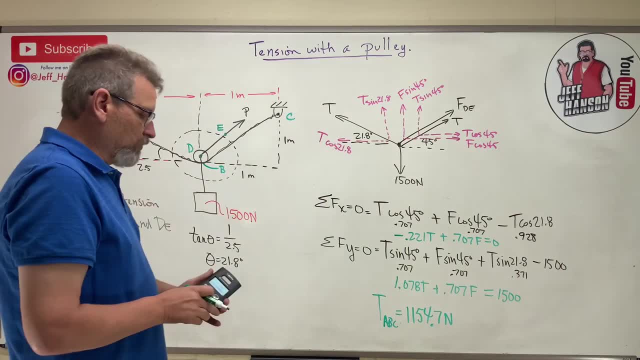 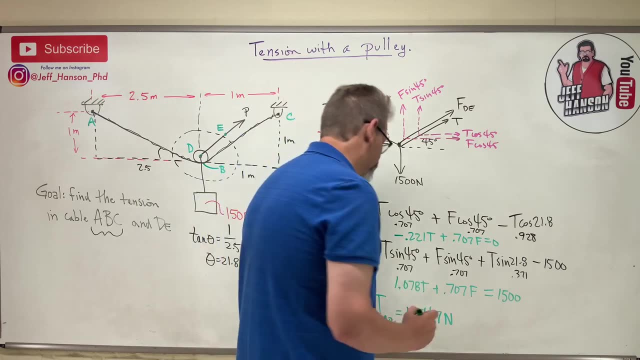 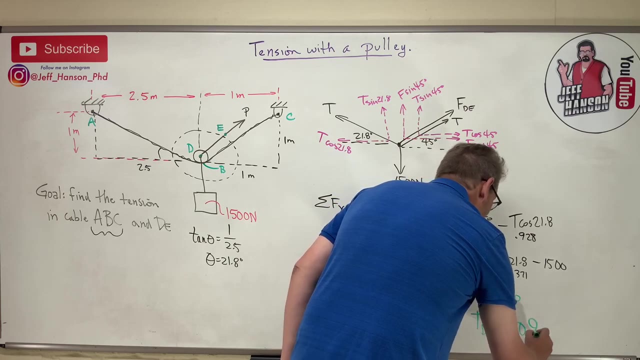 And that's in newtons, okay. And then the next one- it gave it to me also- they gave me the value for f and it's 360.95.. So t d e is 360.95 newtons, okay. 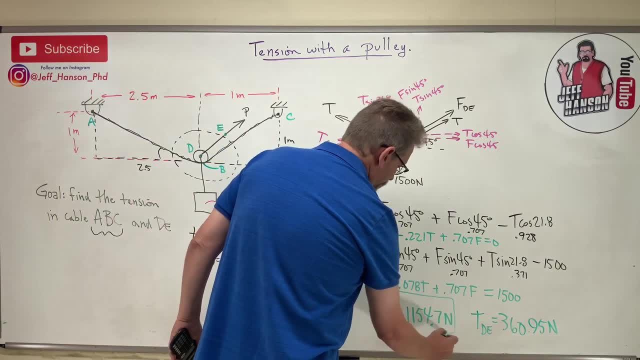 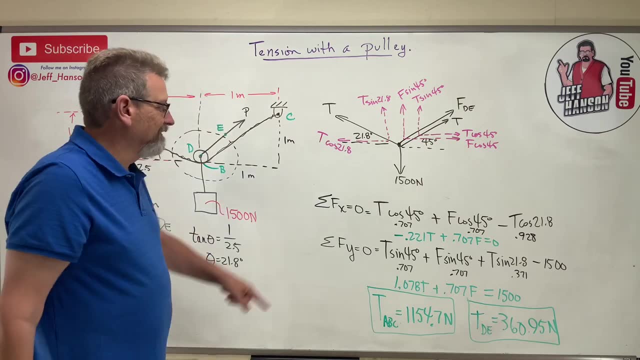 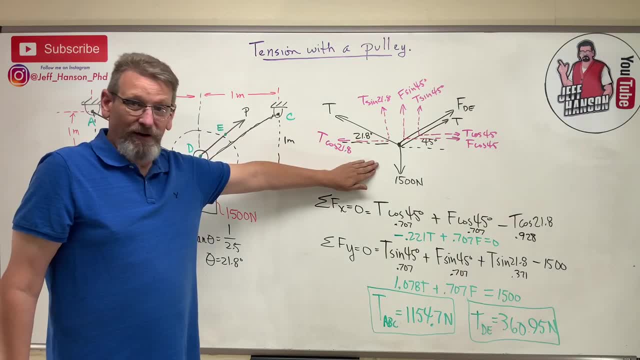 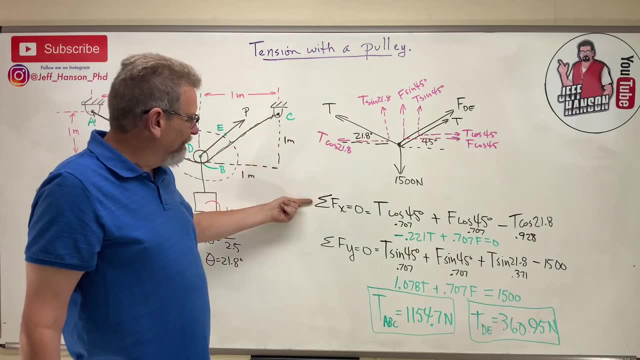 Okay, Okay, Okay, Okay. Well, just please draw big giant clear free body diagrams and label them in color. and then how easy does it make to write these equations if you have that all labeled out, and nice and beautiful. It's so easy y'all. 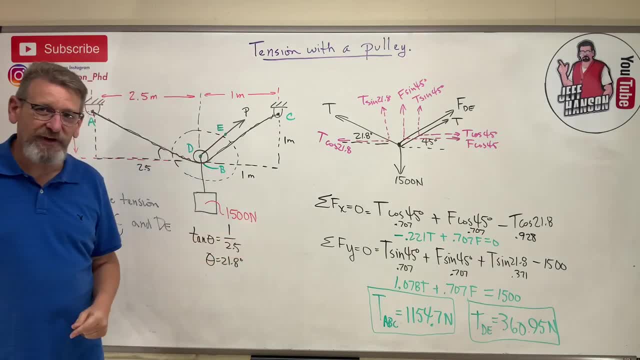 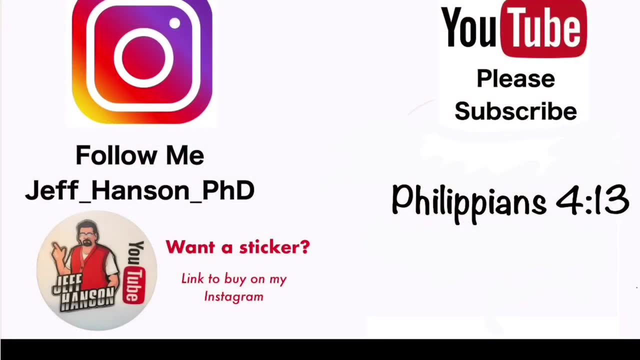 How are you missing this on the test? All right, Let's don't do it anymore. Okay, gang, I'll see you. next problem: We're going to talk about some springs.